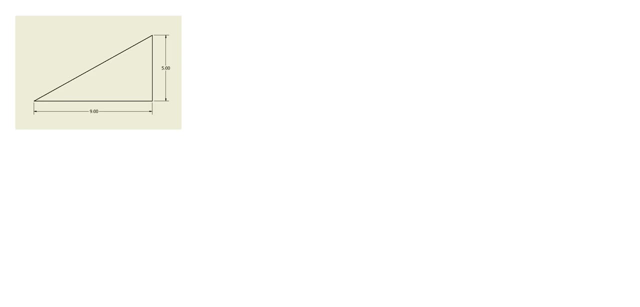 In this particular example, we will take a look at computing the centroid for a right triangle with a height of 5 and a base of 9.. Our x-coordinate, or x-bar, will be given to us using the equation 1-third times the base of the triangle. 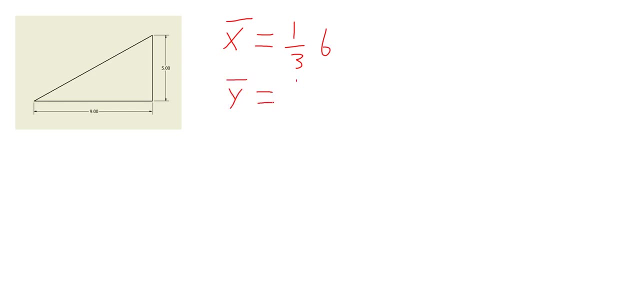 Our y-coordinate, or y-bar, will be given to us by using the equation 1-third times the height of the triangle. In this particular case, x-bar, or the x-coordinate, will be equal to 1-third times 9, or 3 inches. 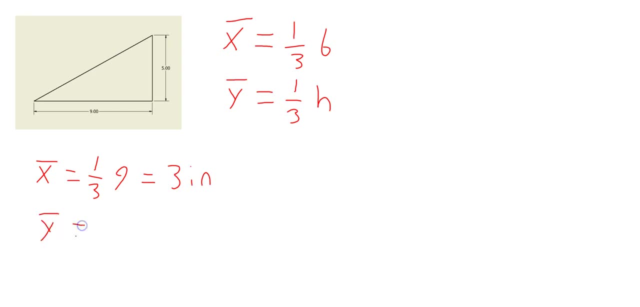 And our y-coordinate, or y-bar, will be equal to 1-third times 5, or 1 and 2-thirds inches. Note that these measurements for the position of the centroid are not the same as the ones we have in the equation 1-third times 9.. 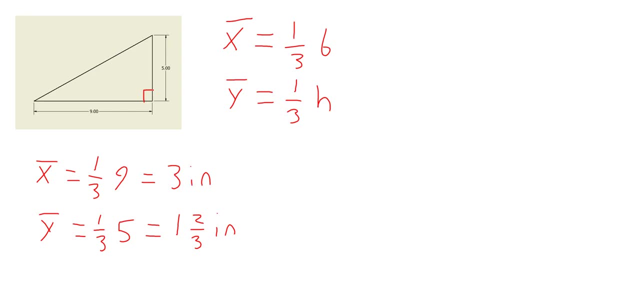 They are in reference to the right angle of the triangle. So what this is saying is that the centroid is located 1 and 2-thirds inches above the right angle of the triangle and 3 inches to the left of the right angle of the triangle. 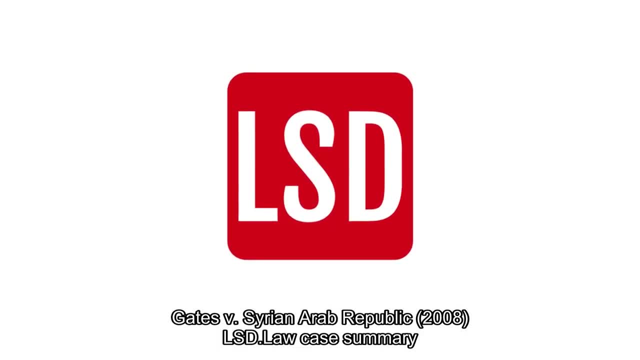 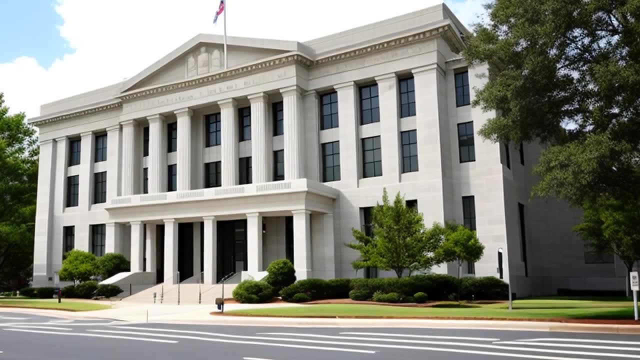 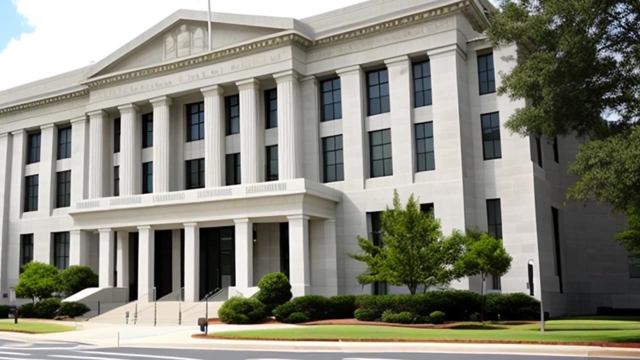 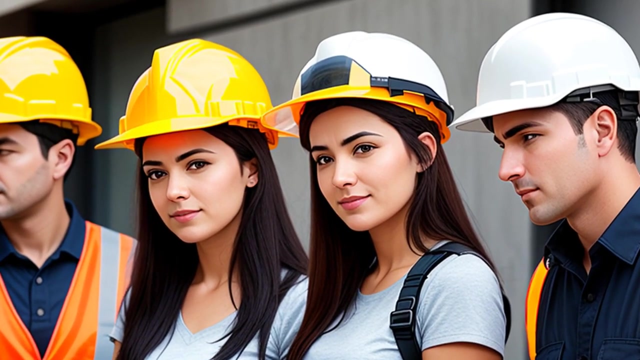 In the 2008 Gates v Syrian Arab Republic case, the United States District Court for the District of Columbia heard claims pertaining to the Foreign Sovereign Immunities Act, FSIA. The families of two civilian contractors, Jack Armstrong and Jack Hensley, filed a lawsuit. 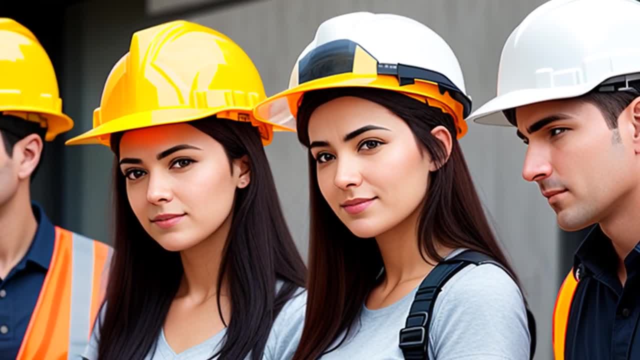 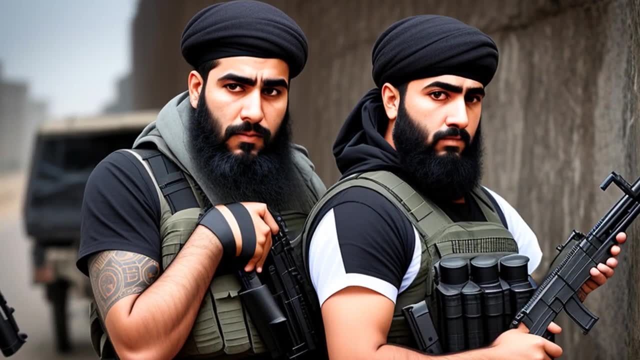 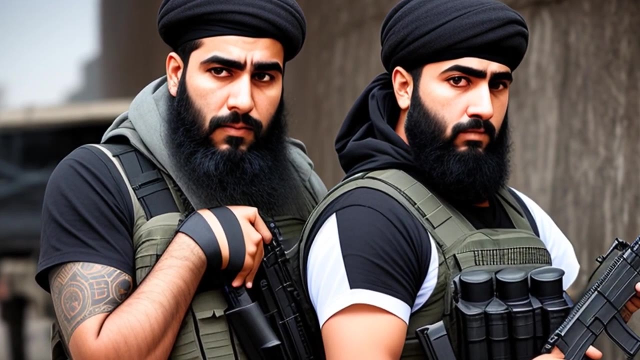 against Syria, its president and military intelligence, for allegedly supporting al-Qaeda in Iraq and contributing to the contractors' deaths. The plaintiffs claimed that Syria provided material support and resources to the terrorist group and its leader, Abu Musab al-Zarqawi, resulting in Armstrong and Hensley's beheadings in Iraq, which were videotaped. 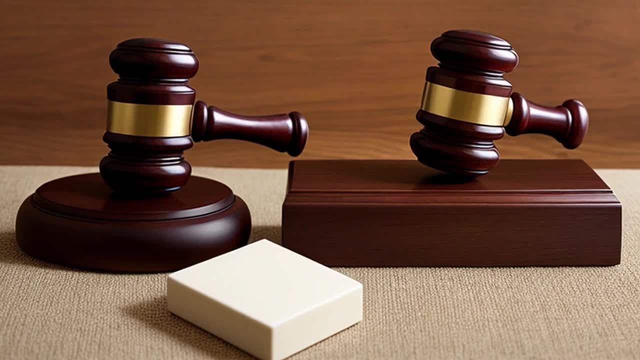 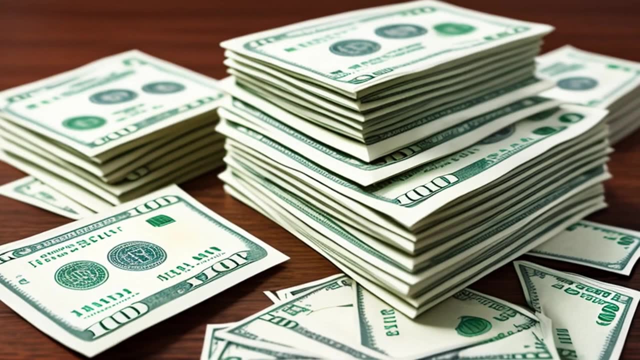 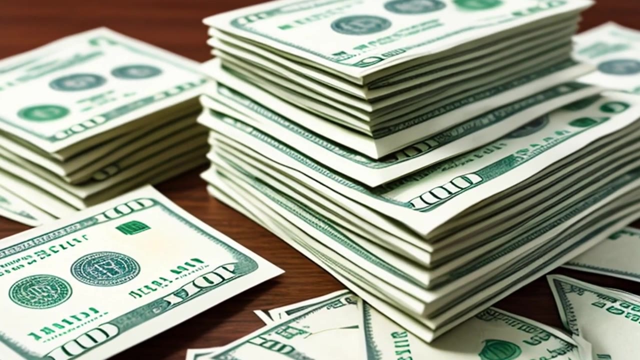 and posted online. The court sought to determine whether the FSIA applied and whether the plaintiffs provided sufficient evidence for their cause of action for damages. In the end, the court awarded the plaintiffs $150 million each in punitive damages, along with a default judgment. for economic damages, pain and suffering. The estates of both victims received economic damages and pain and suffering awards totaling over $1 million each. The ruling signified that US courts will not tolerate states supporting terrorist groups and demonstrated that foreign states can be held responsible for damages in a US court under certain.